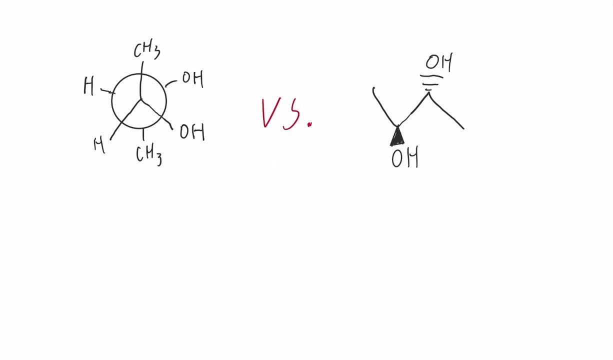 feel free to take a moment to pause and try to do it on your own, Okay, so whenever you're working with different representations of stereoisomers, the strategy I recommend is to redraw one in the other form. Newman projections are just skeletal structures seen from a different point of view. 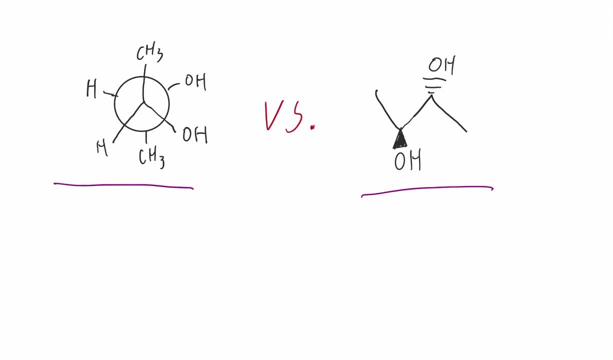 and I'll color code it so you can see which carbons represent each other. So this carbon that I'm coloring blue represents this carbon on the simple skeleton structure and the big circle on the back represents this carbon and the simple skeleton structure. Now all the other projections you see on the Newman projection. 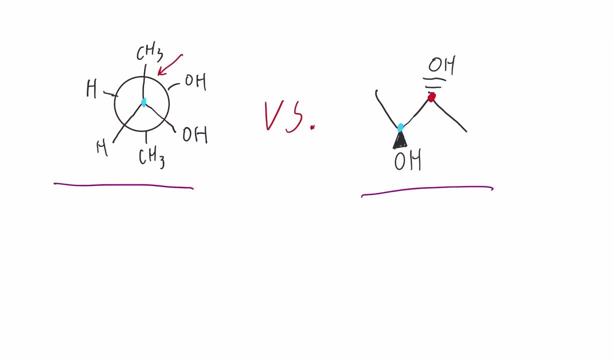 are the substituents of those two carbons. So this OH group represents OH group here and the same way that this OH group represents the OH group on the back carbon. So to recreate the Nguyen projection as a skeletal structure, we're going to redraw. 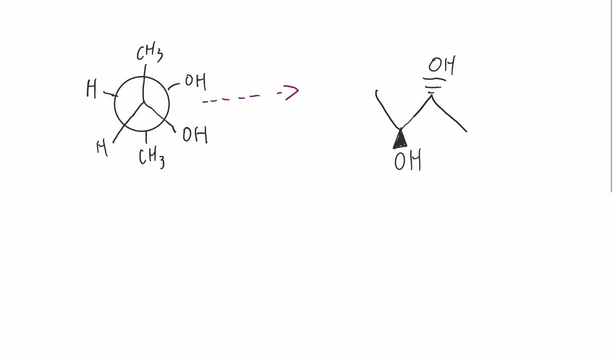 it as if we are facing it from this direction. From that point of view, you still have your front carbon and your back carbon, And then, coming off of the front carbon, you have a methyl group coming up, And coming off of the back carbon, you have a methyl group going down. 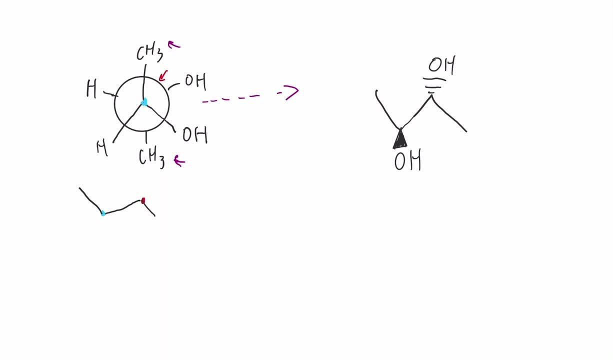 Okay, So that's the carbon structure And that more or less aligns with the carbon structure on the structure we're comparing it to. But now let's fill in the other substituents. Once again, we are facing this Nguyen projection from over here. 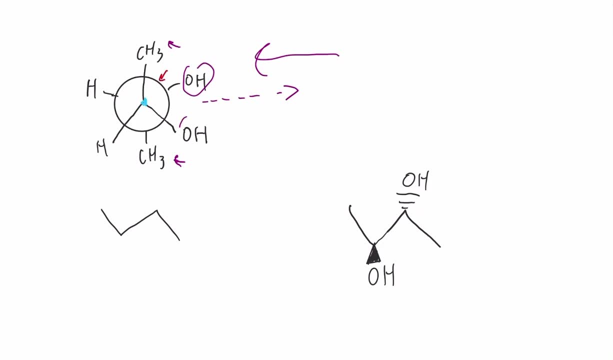 So we need to draw these OH groups as if they are oriented in the way that we see them, Where, if we're facing them from this right side, they would both be coming out towards us, which means that when we redraw it, we would see them both on wedges. 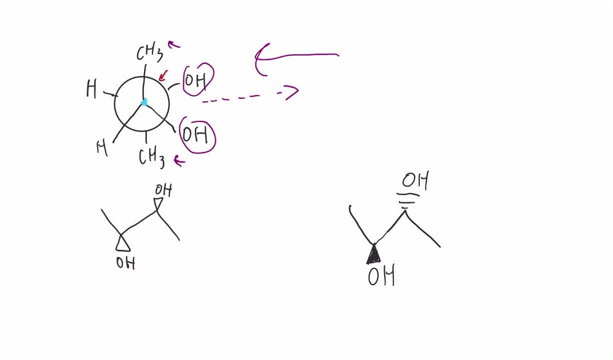 Now we can just compare these two. PIO2 is even比F choice V and PIO2 is argue V. Now we can just compare these two. So in doing that, we can quickly see that each of these structures has two chiral centers. 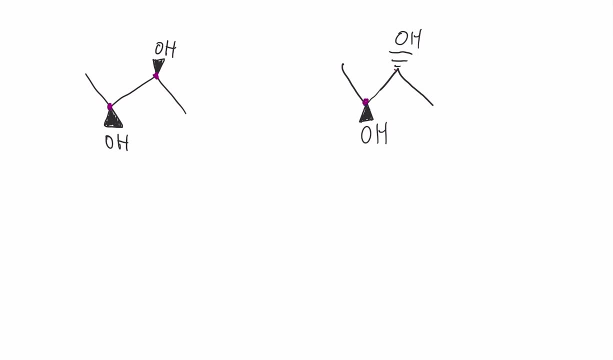 PIO2 is even比F, PIO2 is even比F, And that one of them is exactly the same, but one of them has switched orientation, which means that these two structures are in the same new form. PIO2 is even PIO2.. 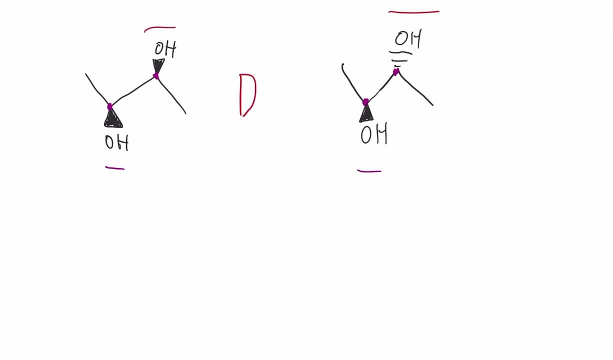 15,000.. 15,000.. 15,000., 15,000. 15,000. 15,000. 15,000.. are diastereomers. Let's do another, one of those for practice. Give this one a. 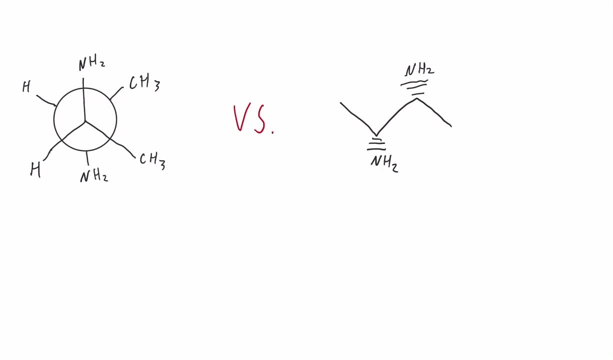 shot. Okay, so we're gonna implement the same strategy as last time by redrawing the Newman projection, but it may be a little bit trickier because the methyl groups aren't just neatly facing up and down to line up perfectly with the methyl groups on the skeletal structure. However, this bond, this single bond, 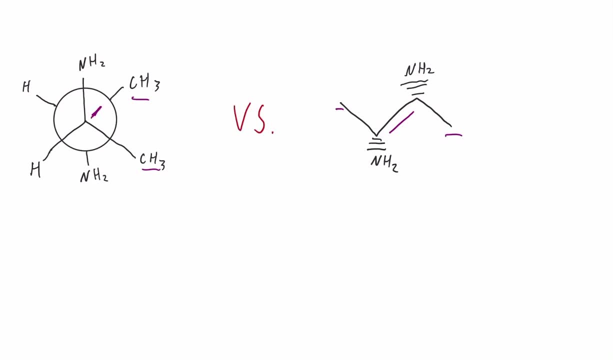 between these two garpins, which is also seen like between these two, can rotate freely So we can redraw the Newman projection after rotating about that bond. So we're going to physically take this carbon in front and rotate it up to the top and we're gonna rotate that entire front carbon, that entire front. 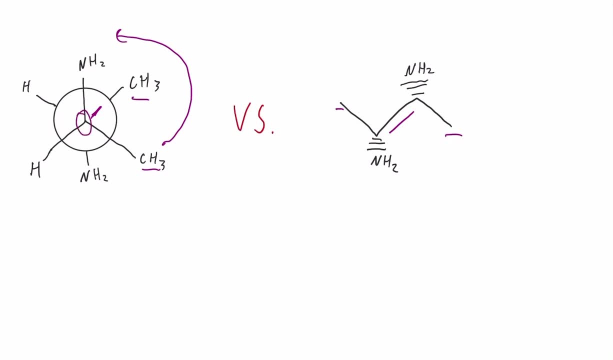 section with us. So it'd look like this: If we move the methyl group up top, we're also rotating this NH2 group down, So this- Th ev Mt� would be here and it would keep rotating, so the hydrogen would be here. This is CH3. 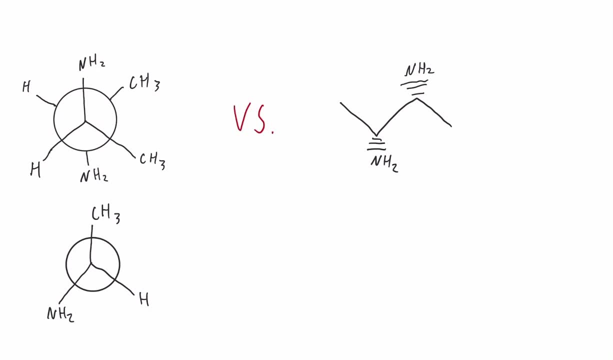 We can also rotate the back carbon to a similar effect, where we're going to rotate this methyl group down to be facing at the bottom. If we did that, we'd have the methyl group here. We would continue to rotate that with this NH2, so the NH2 would be up here and the hydrogen would rotate. 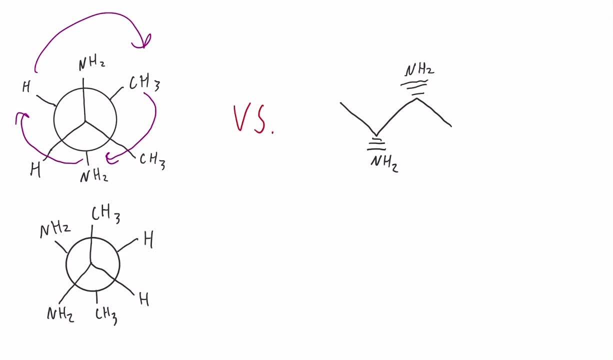 up here Now. this Newman projection is much easier to redraw, and we're going to do so as if we are facing it from this direction Once again. we have our carbons in front and in back, with a methyl group coming up from the front one and a methyl group going down from the back one. 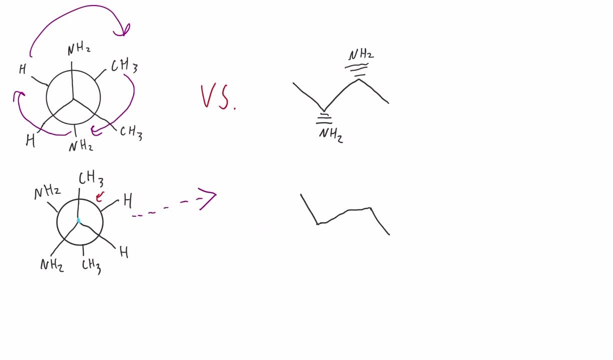 Now we just need to add on the other substituents, with those being the NH2 groups. When we're facing from the right, we can tell that this NH2 on the front carbon would be facing away from us. so that would be on a wedge or on a dash, excuse me. 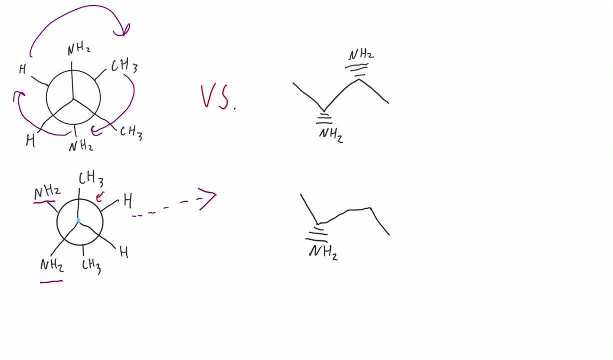 and same goes for the NH2 on the back, carbon, which would also be on A. Now we just need to compare these two and it really should not be too hard to tell that these two are exactly the same. so they are identical, Nice. Another alternative structural representation that you'll commonly see is the chair conformation for 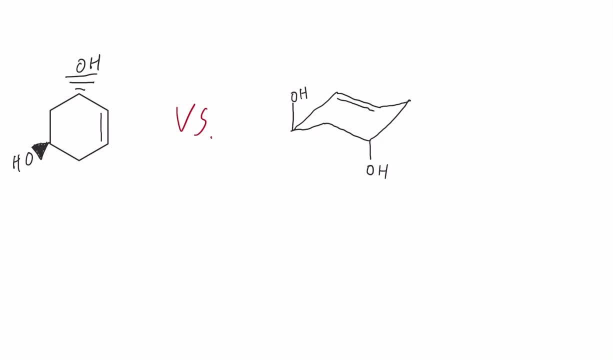 cyclohexane. In this case we're going to go about it the same way, by redrawing it in the form that's easier to work with. but again, feel free to pause to try to give it a shot on your own first. Okay, so I think these are a little bit easier to work with than Newman projections, because 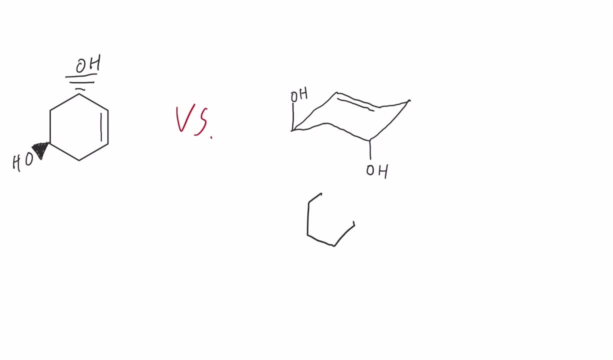 they pretty much directly translate to the general cyclohexane that we work with. So we're going to draw on the double bond because there is a jumble bond represented here and now we just need to add in the substituents. We can note that the way from the way that we're looking at it, one carbon over counterclockwise. 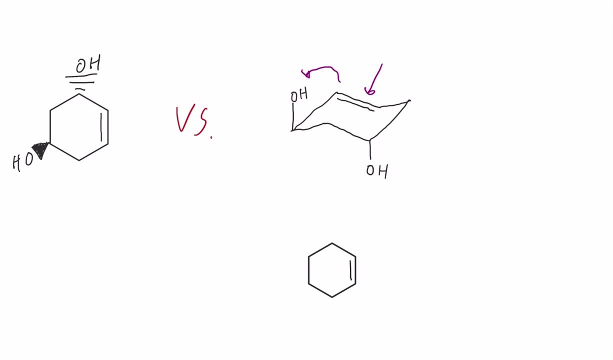 from the end of the double bond there is an OH group and also there is one, two carbons clockwise. from the end of it there is another OH group, one, two, another OH group here. Now our only concern is the stereochemistry of those OH groups. 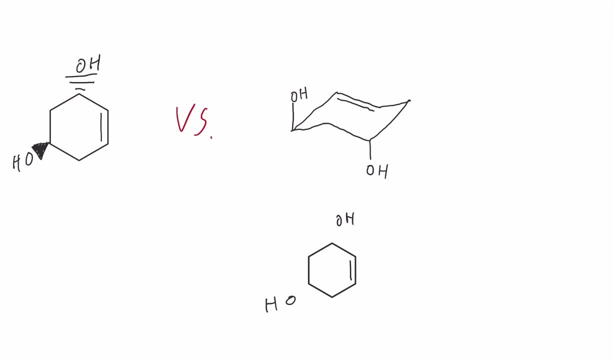 The key insight is that chair conformations are drawn under the assumption that you are facing them from above and not from below. So this OH group is also this one, when facing from above would be coming out towards us, so it would be on a wedge, and this group would be facing away from us, so it would be on a dash. 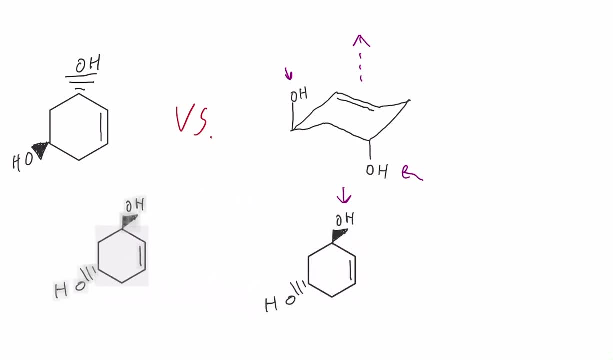 Now that we have this structure redrawn, what we need to do is compare it to this. Okay, so we can compare these in two ways, and we're going to do both to get this check. First is we identify that there are two stereocenters. there are two chiral centers there. 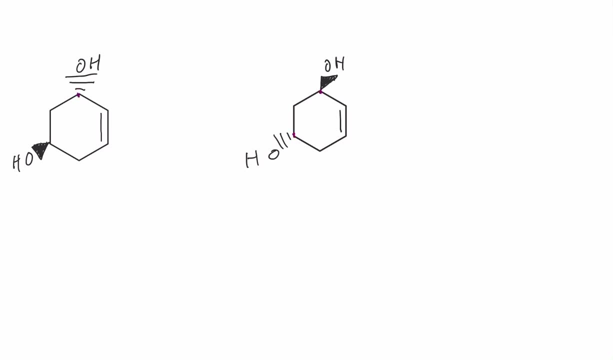 there's carbon on each, there's those two chiral centers, and then we're going to compare it to this. Now that we have this structure redrawn, what we need to do is compare it to this, And then we can tell from this oriented like, oriented this way, how many of them have flipped. 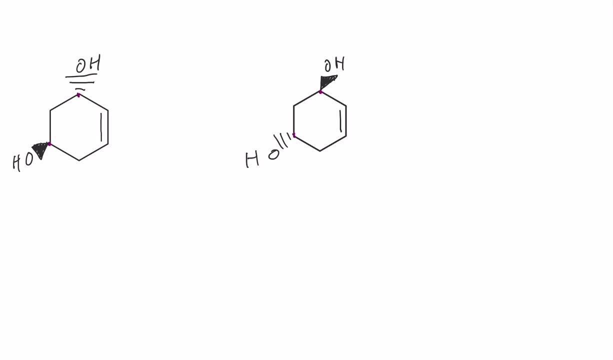 how many of them have stayed the same? And we look at the first one. it goes from a wedge to a dash, and the other one goes from a dash to a wedge, which means that both of the stereocenters have flipped, which means that these are most likely enantiomers. 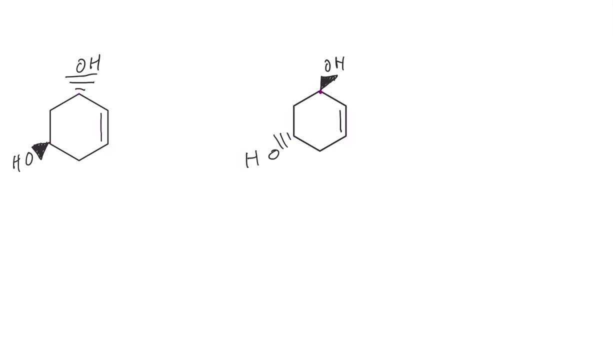 The other way we can confirm this is with the mirror image test. so I'm going to draw the dotted line down the middle of the page and we're going to imagine that that is a mirror. You'll recall that enantiomers, by definition, are non-superimposable mirror images. 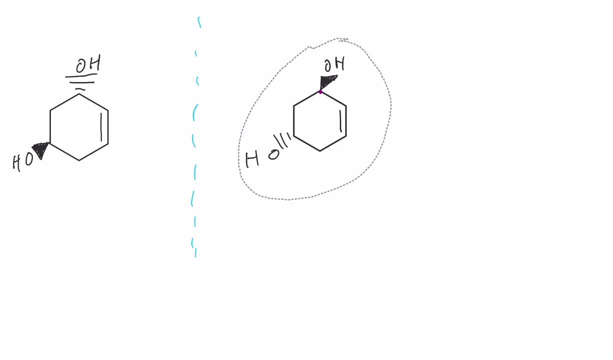 We can confirm that these are not superimposable simply by trying to superimpose them. We can drag this one over and we'll see that, while the double bond is in the same place, we can never have these aligned. We can also see that, as I was saying, these can either be facing the other side the line. 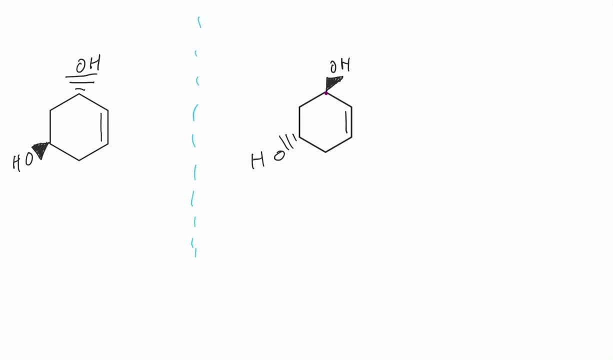 because the OH, the substituents, are facing in opposite directions, So these are super non-superimposable. Now the question is: are these mirror images? So now, if you think about when you're facing a mirror, things that are close to the mirror, 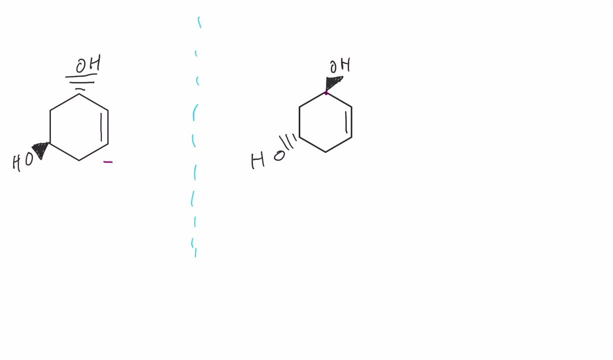 appear close on the other side. so this double bond here is the closest thing to the mirror, so it should be also the closest thing to the mirror on the other side, but in this case it's all the way over here. So what we're gonna do in order to make this: 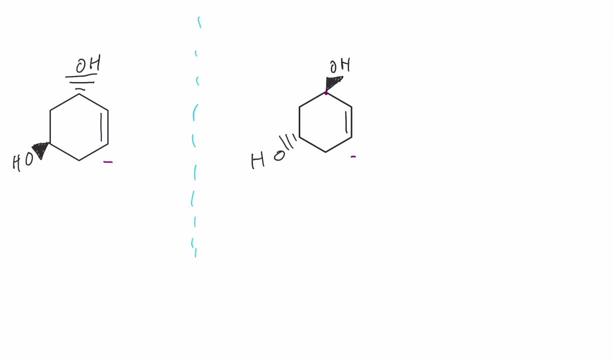 to see if this is a mirror image, is we're going to flip this over along like this plane, almost like a pancake. We're just gonna pick up this double bond and we're gonna flip it over onto the other side like a pancake. 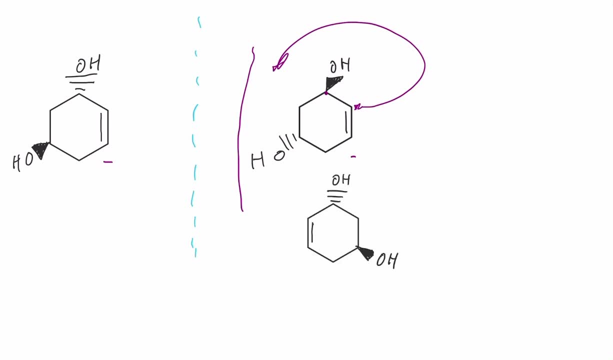 And what that will give us is gonna look kind of like this: Okay, so we're gonna raise this, because it's the same thing as that, just flipped And we're going to move this up, And now we can compare these two to see if they are mirror images. 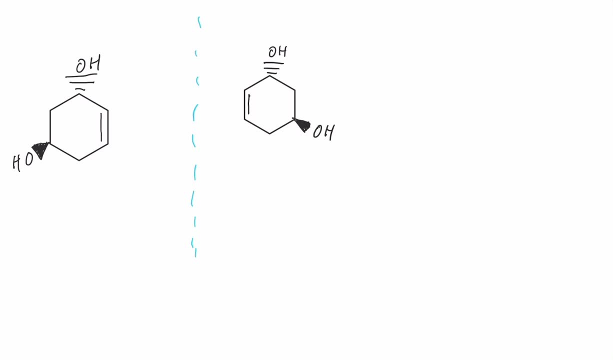 because we already confirmed they're non-superimposable, And now we can see that kind of like how, in a mirror, these things align with: the things that are close are close. on the other side, The things that are facing out are facing out. 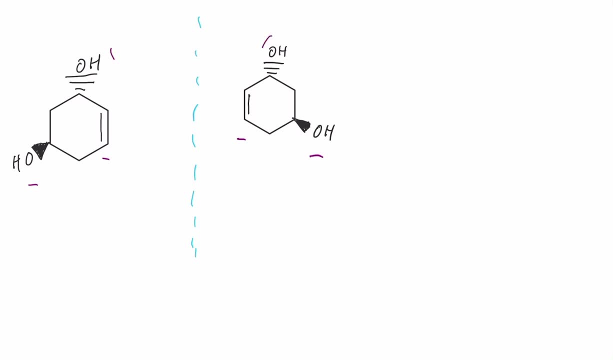 On the other side. the things that are facing in are facing in on the other side. So these things are mirror images and they are superimposable or non-superimposable rather, So they are enantiomers. Okay, let's practice with another one of those. 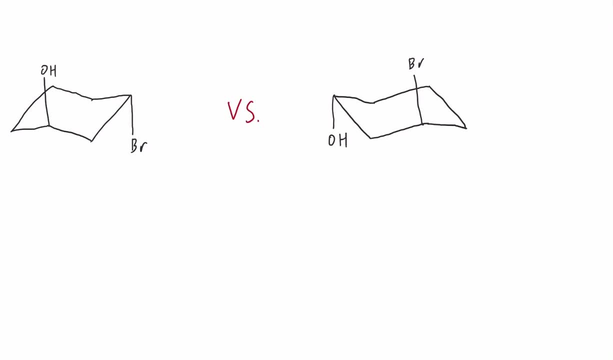 Pause it and give it a try. Okay, we're gonna do the same thing as last time, like with redrawing the share confirmations, It's just that there's two of them this time, So if you start with the one on the left, 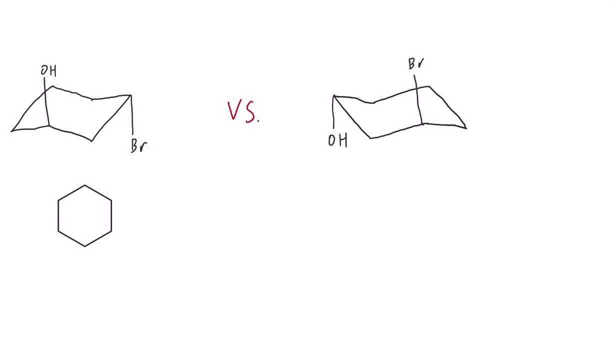 we have a cyclohexane and we have a bromine going away from us. It's going down, but since we're looking at it from above, that bromine is going away from us, There's no double bond here, so we can draw them really in any position we want to. 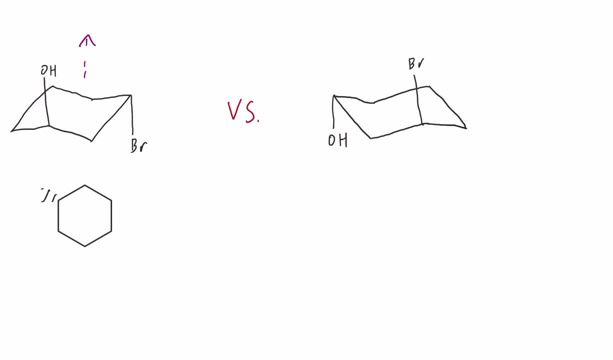 So I'll just draw the bromine here. They just need to be in the same spot relative to each other. So we have an OH group that's coming up, It's coming towards us And that OH group is two carbons away, going clockwise. 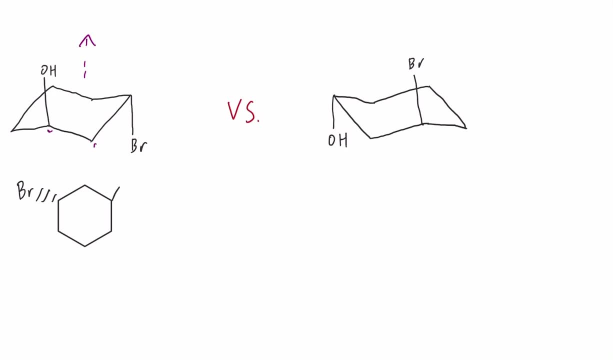 which means that it would be here. We have an OH group coming up towards us. Now let's draw this one on the right. We once again have a cyclohexane. This time we have a bromide going up, which means it's coming towards us. 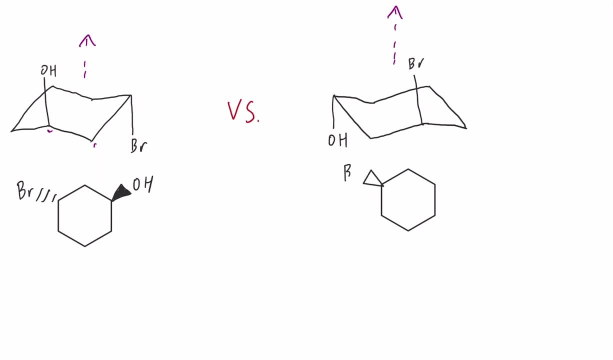 So we also have going two carbons in the clockwise direction, an OH going down, which means it's away from us. So now that we have our two structures simplified, we can just compare these two, Since we already have them aligned like this. 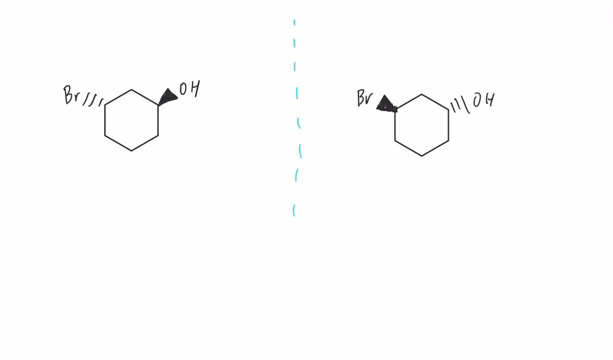 I say we start with our mirror image tests for this one. They're already aligned in terms of their general orientation, but are they superimposable? No, You can see that the, The substituents are in the right position, but they overlap with wedges and dashes instead of being on the same spot. 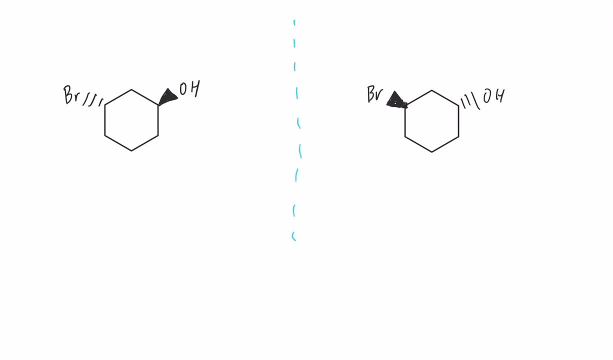 So they're non-superimposable, Are they mirror images? It may be harder to see this way, but you may be able to see this If the mirror was in the line of the page, like it was in the plane of the page, like, instead of having this vertical mirror we had, like, the screen itself were a mirror and we were holding this one above the mirror. 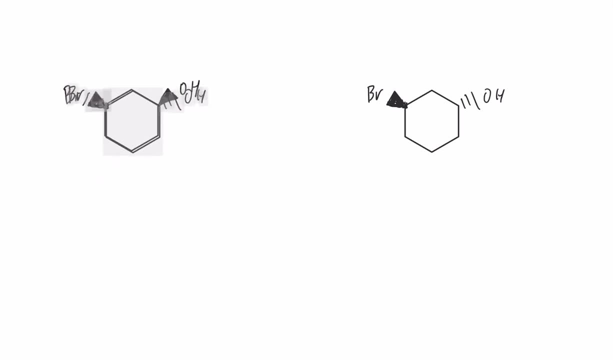 You could see that these would be mirror images, because what is above what is facing towards us, which would be far away from the mirror? If the mirror is on a dash, it would be far away from the mirror on the other side, and vice versa. 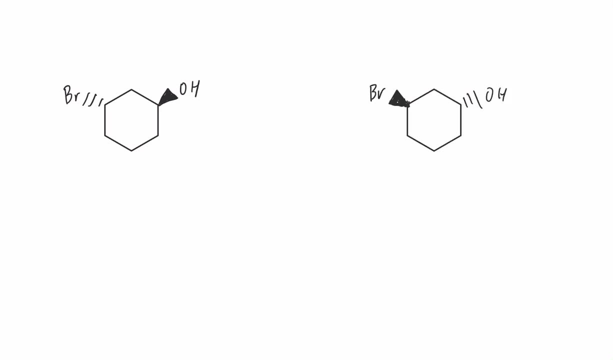 But that might be harder to see. So what we can do is something similar to last time, where we still use a mirror that's like drawn vertically in the page, But we just flip one of these like a pancake. We'll flip this one like a pancake. 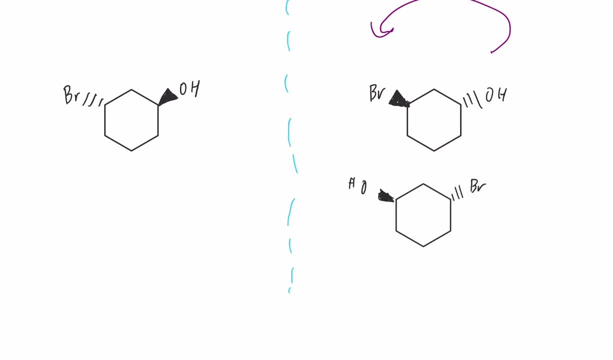 And that'll look like this, And now we can compare these to like we did Last time with the mirror, to see if they are mirror images. What is facing towards us is facing towards us. That may come from facing away, facing away. 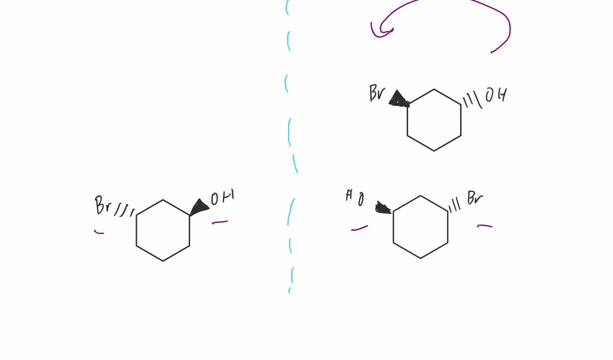 What's close is close, What's far is far. Those are mirror images and they are non-superimposable, So they are enantiomers. The other way that we can check. We can go back to comparing these two, And we can do it by identifying the stereocenters. 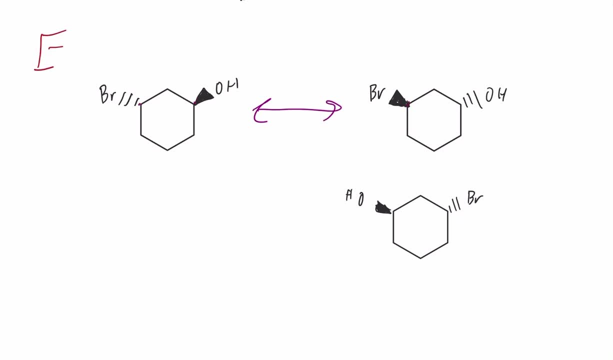 There's two of them, One, two, One, two, And we can see how many of them flipped: The bermide went from being on a dash to being on a wedge And the OH went from being on a dash or a wedge to a dash. 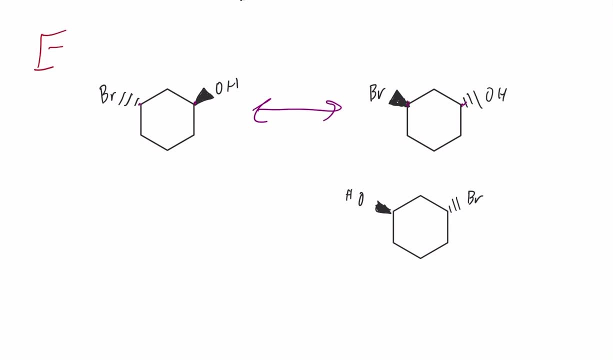 So they both flipped, which means that all the stereocenters have changed, Which means that they are definitely enantiomers. Moving on to the next problem: Are these enantiomers diastereomers or identical? Okay, so for problems like this one where you have multiple stereocenters, 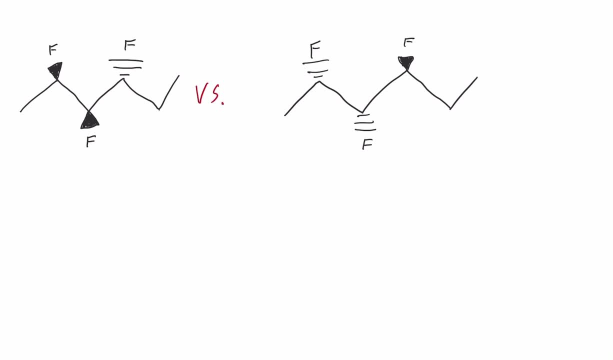 And as that number keeps increasing, it may be easier to go through the method of identifying each stereocenter and its orientation Rather than going straight for the mirror image test. So let's do that. Let's identify the stereocenters. 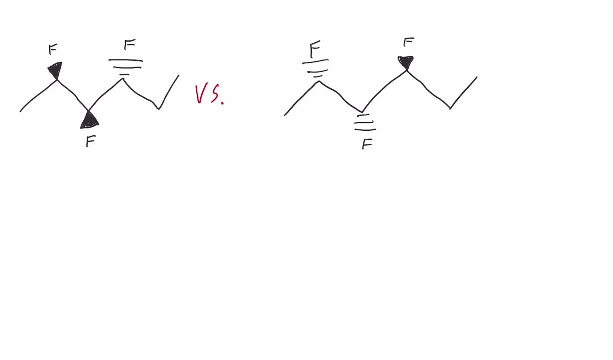 And then assign either R or S to each of them And see how they compare. So for this first one, on the far left, If we're assigning priority, Fluoride is one, This would be two, This would be three, Because the top three priorities 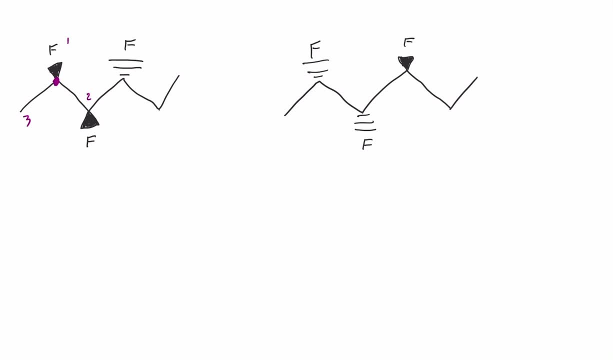 Are facing towards us And the fourth priority, which is the hydrogen, is facing away. We can simply count around One, two, three And because that is going clockwise, We can call that R. Now let's move on to this chiral center. 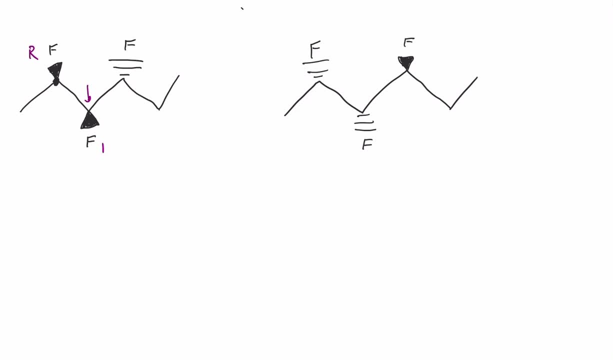 This would be the first priority. The second priority may be trickier, Because you both go to a carbon That is bonded to a fluoride, But the one on the right has an additional methyl group tail at the end, Which matters when everything else is identical. 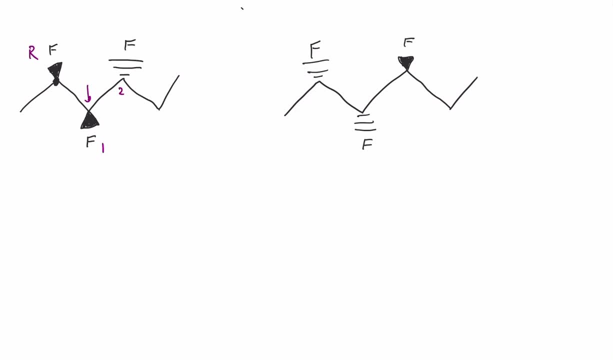 Which means that this is the second priority And this is the third priority. So we can count From one to two to three, And because that is counterclockwise, We call this S. Now for this last one, We can do the same thing. 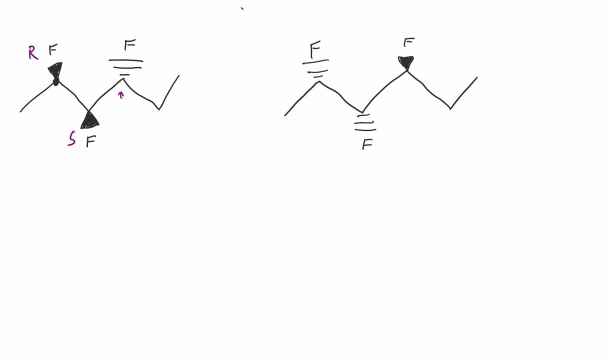 This is first priority, This is the second priority, This is third priority. Now we're going to count around One, two, three Through the priorities, And that is counterclockwise, Which would give us S normally, And that is counterclockwise. 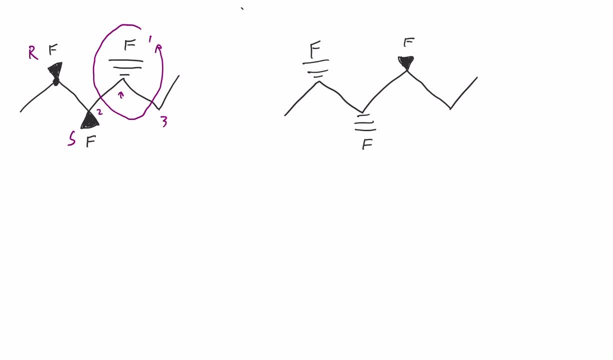 And that is counterclockwise, And that is counterclockwise, Which would give us S normally, But because there is an implicit hydrogen, Like the fourth priority is coming towards us, Because the fourth priority is coming towards us, We just take that orientation. 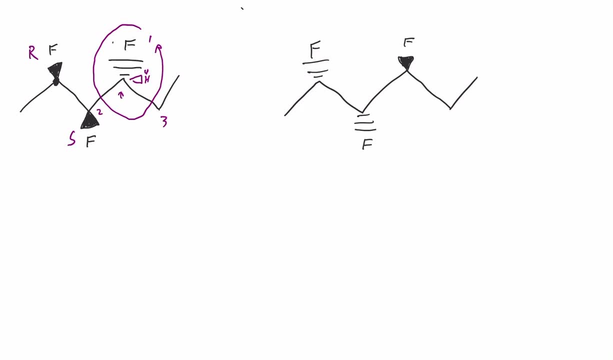 And we flip it. So instead of S, this would be R. Now let's move on to the structure on the right. Let's start with this carbon. This is first priority, Second priority And then third priority. We count around One, two, three. 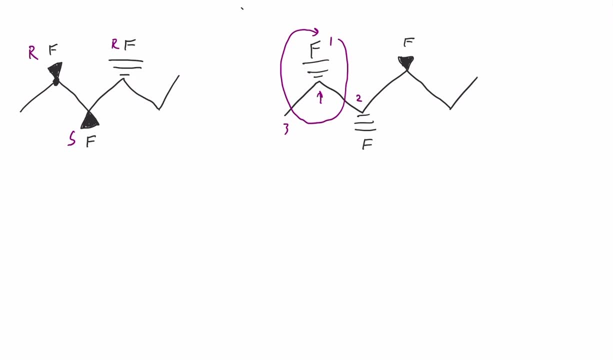 That is clockwise, Which would be R If the F was coming towards us. If the F was coming towards us Because it's going away from us, The fourth priority is coming towards us, So we have to flip it, Which makes this S. 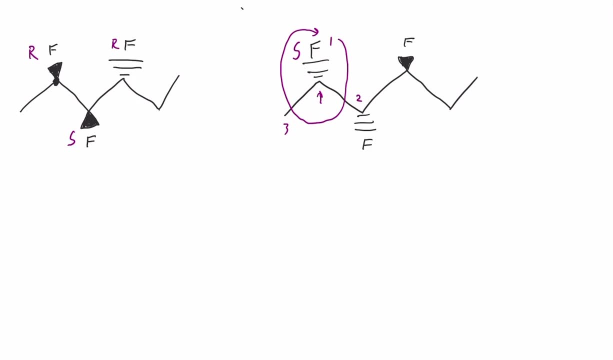 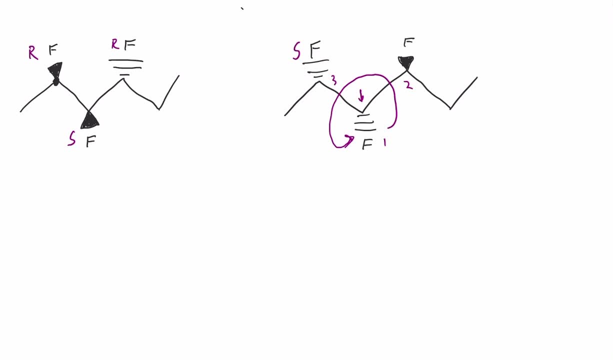 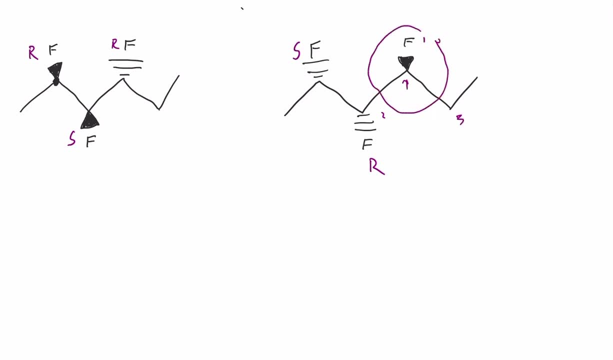 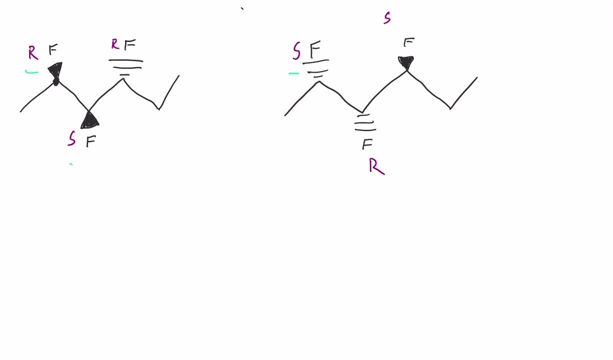 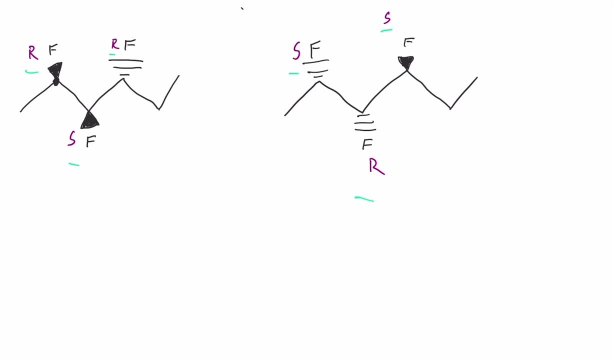 Meaning that all three chiral centers flipped their orientation, And that tells us, because every single one changed, that they are enantiomers. Now, here's the last problem. Pause it and give it a shot on your own. Okay, let's approach this one the same way we approached the last one, by starting with assigning R or S to each stereo center. 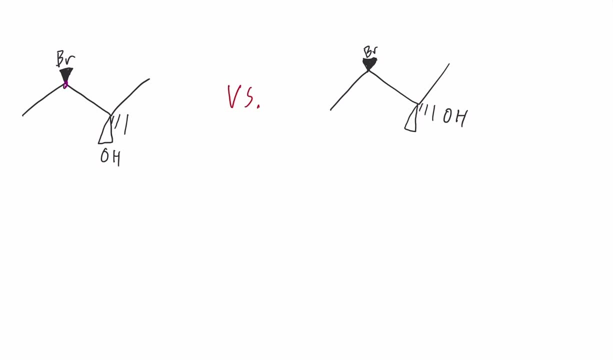 Let's begin here. The bromide is the first priority, This is the second priority And then this is the third priority. We can count 1,, 2,, 3 in the clockwise direction. The hydrogen is facing away from us, So this is R. 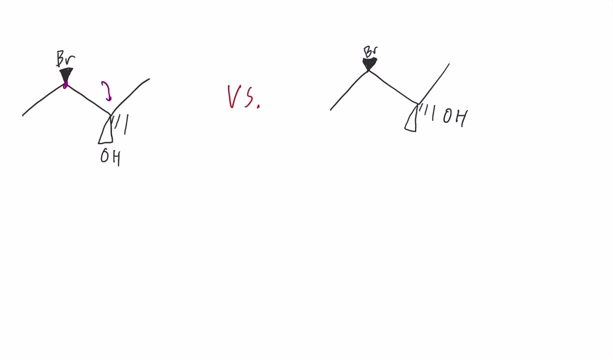 Now moving on, we'll go to this card. If we try to do the same thing here, we'll run into some issues. This is clearly first priority. This would be second priority, But what is the third priority? Both this projection and this wedge just represent methyl groups. They're just CH3s. 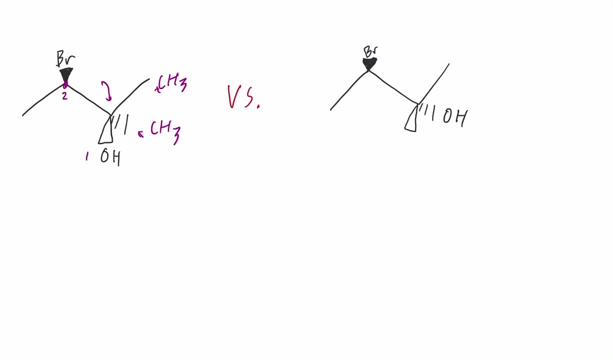 Meaning that they are identical, like these two groups. And we know that for a carbon to be chiral, it has to be attached to four unique things. So because this carbon is bonded to two methyl groups that are the same, this is not chiral. 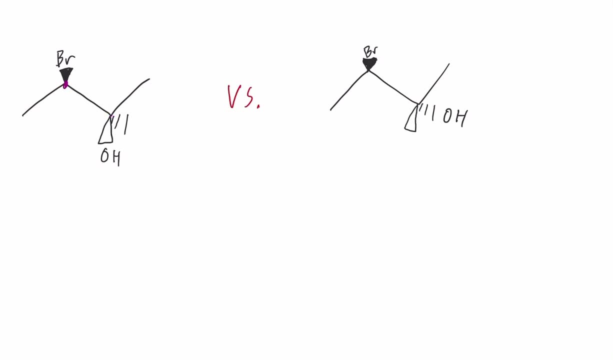 So that tells us that there is only in these structures, there is only one chiral carbon, And it's this one that I highlighted in purple, Because the other one is not chiral. It can rotate freely. In fact, this is just the same thing as this, but rotated so that the OH group is facing back instead. 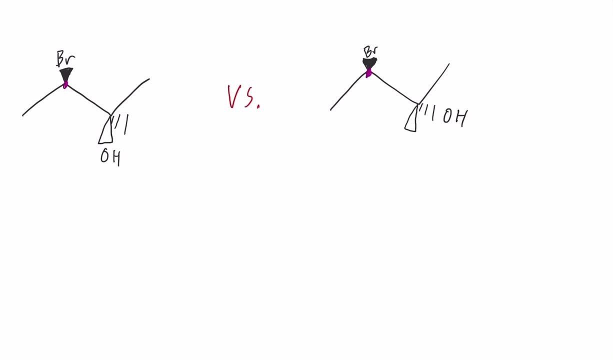 And this is a way that professors could easily try to throw you off, just by drawing a methyl group in two different ways Or doing something similar to this. So it can be really helpful going through each carbon that you believe is a chiral carbon. 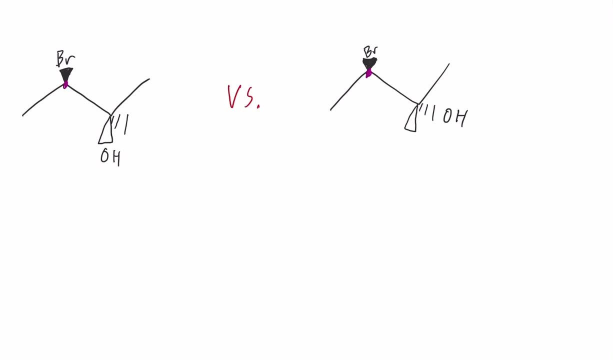 So it can be really helpful going through each carbon that you believe is a chiral carbon. So it can be really helpful going through each carbon that you believe is a chiral carbon And assigning R or S, because you would catch those types of mistakes by doing that. 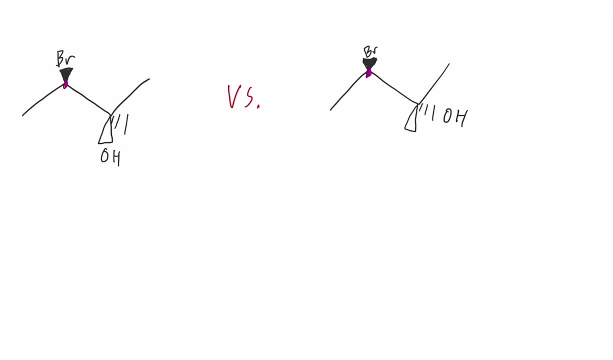 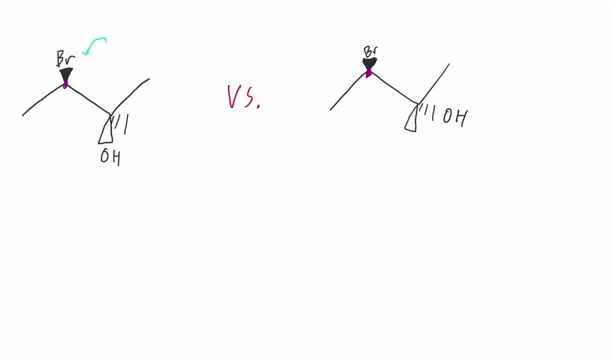 And assigning R or S, because you would catch those types of mistakes by doing that. So we only have one chiral carbon and it did not change at all. So we only have one chiral carbon and it did not change at all. 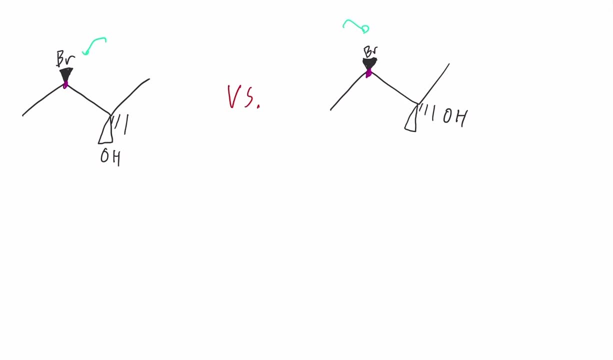